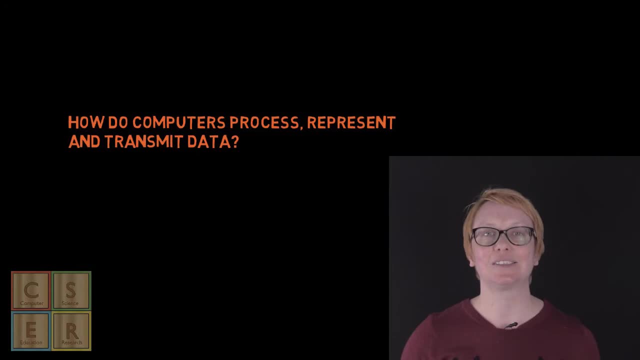 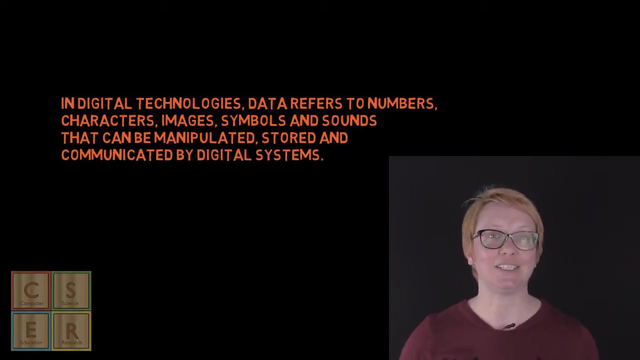 In a general sense, data refers to a collection of facts, symbols or numbers. In digital technologies, data refers to numbers, characters, images, symbols and sounds that can be manipulated, stored and communicated by digital systems. One way to explore how computers process and transmit data is to look at how we, as humans, transmit and process data. 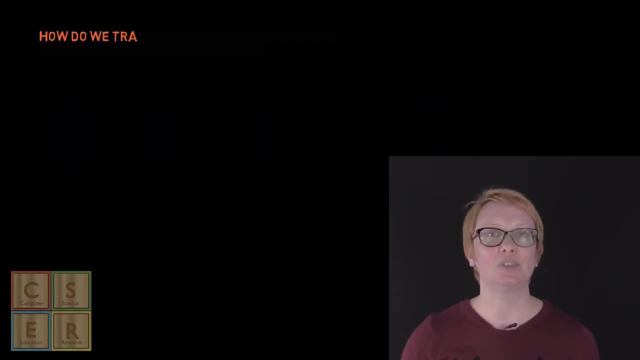 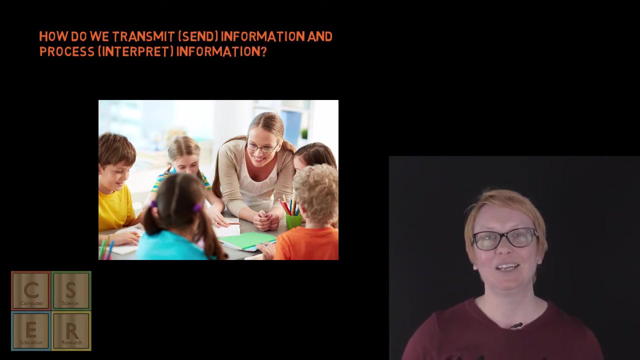 Exploring voice tone, verbal and non-verbal cues, words to transmit and to process. we look at body language expressions, listen to tone and what the person says. But what if a condition was changed? What if we weren't able to speak? 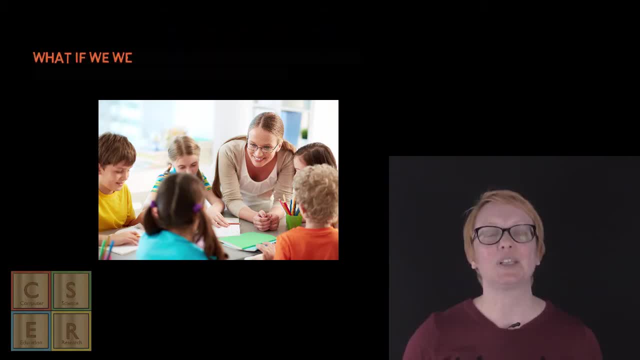 What if we couldn't speak to or hear one another? How would children transmit a message to one another? Perhaps in the class, change a condition such as not being able to speak or write, and have students think of ways to transmit a message. 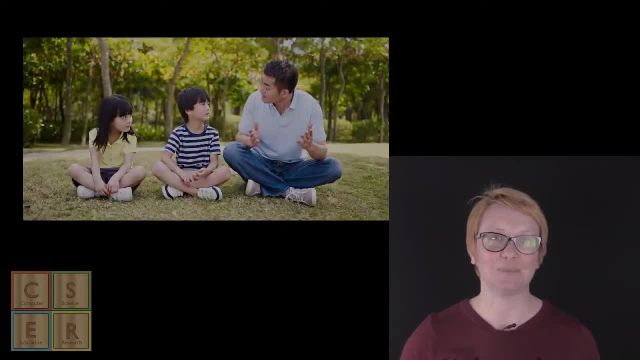 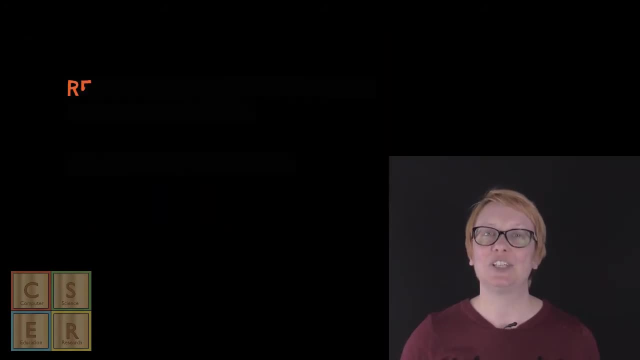 Pair students up and give them time to figure out a plan for their new system. Either give them a random message to send or ask them to create a message. Reflect and share ways of communicating. What worked best and why. What made it difficult? 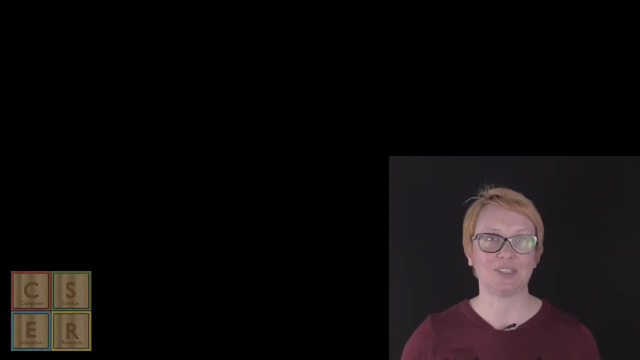 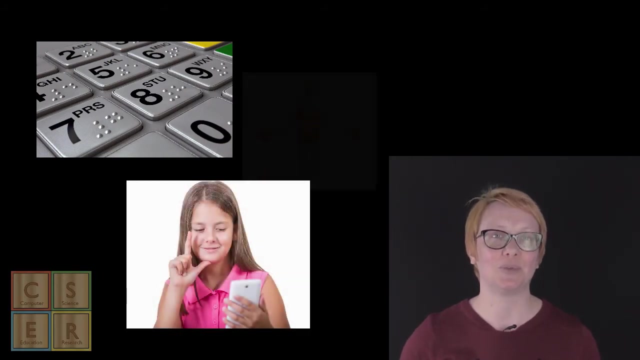 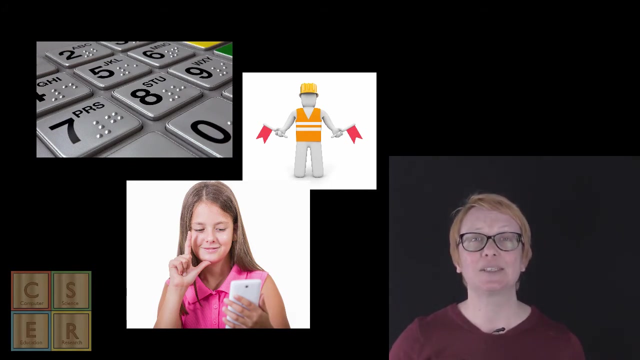 There are different types of coding systems that are used to transmit messages. Let's have a look at some examples, including braille sign language and flag signals, such as those used at airports, or the semaphore system. These systems have been created for particular purposes and work with certain limiting factors or existing factors. 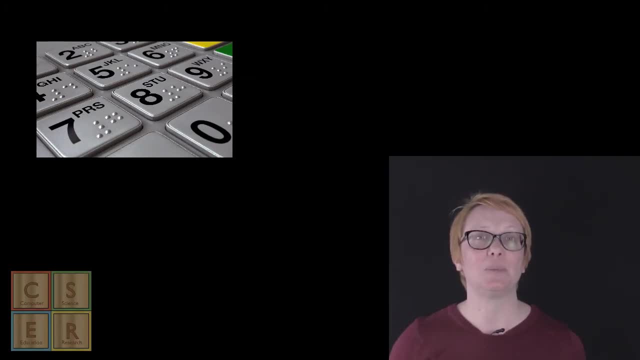 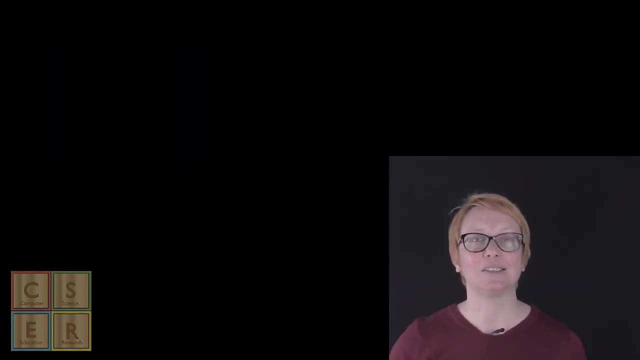 For example, braille is a configuration of raised dots used where people cannot see clearly but are able to use the sense of touch to feel the message being conveyed. Sign language or flag systems work with the ability to convey a message using visual mechanisms. 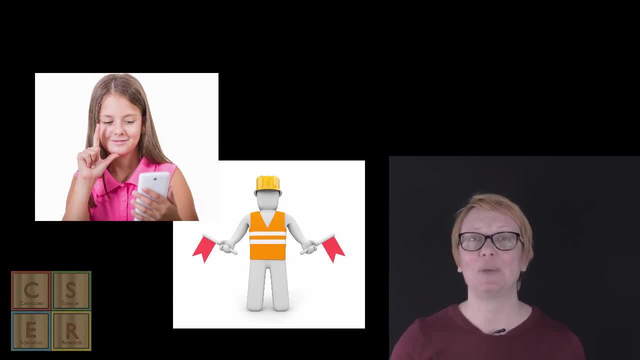 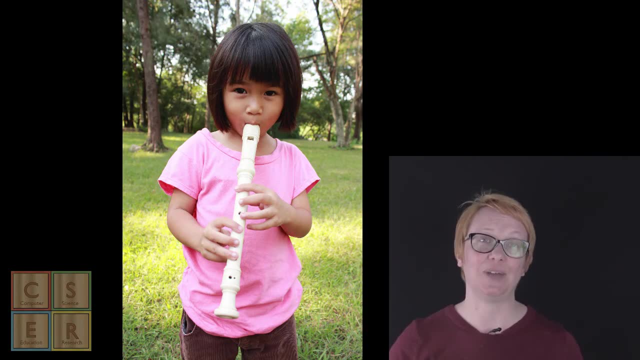 There are also other ways, such as through the sense of sound, perhaps by the use of whistles or by voice. The text you are able to read on the screen is one system that humans use to convey information. Computers are electronic machines. 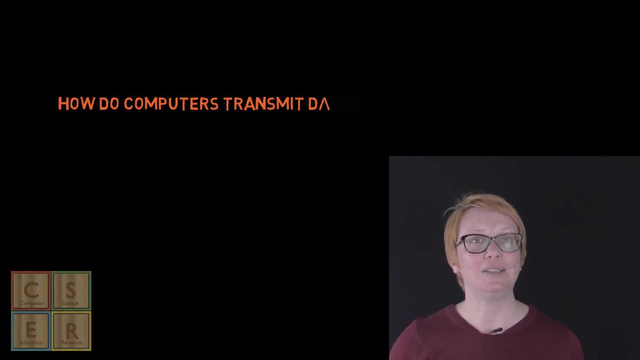 The computer uses electricity, not mechanical parts. except for some components like the disk drive for data processing and storage, Electricity flows through switches. If the switch is closed, the electricity flows. If it's open, it doesn't flow. To process real-world data, for example a text message. we need a way to represent data in switches.